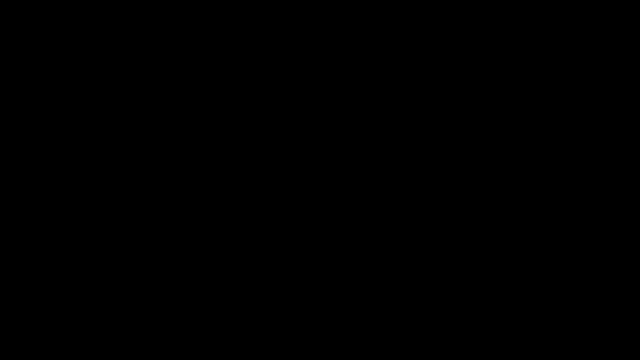 In this video we're going to focus on calculating percentages without the use of a calculator. We're going to do it mentally and then we'll confirm our answer with the use of a calculator. So here's the first question: What is 15% of? 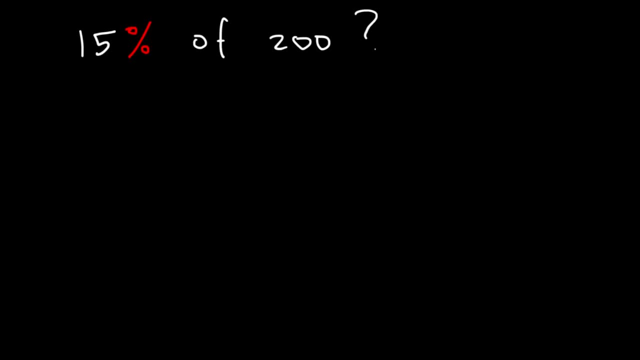 200?. How can we find the answer to this question mentally? Well, first ask yourself: what is 10% of 200?? To find 10% of a number, simply move the decimal one unit to the left. So 10% of 200 is 20.. Now, if 10% of 200 is 20,, what is 5% of 200?? 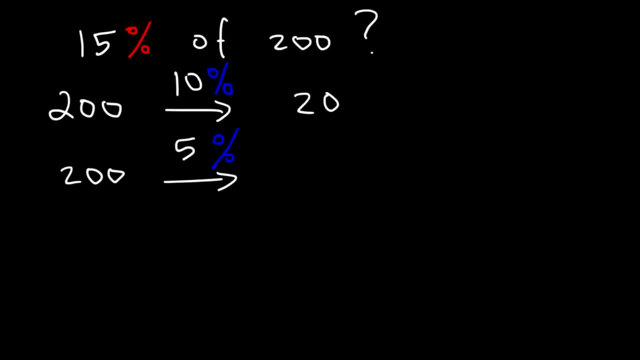 5% is half of 10%. So what is half of 20?? Half of 20 is 10.. So now, with this information, how can we find out the value of 15% of 200?? Well, since 10% plus 5% adds up to 15%, 20 plus 10 must. 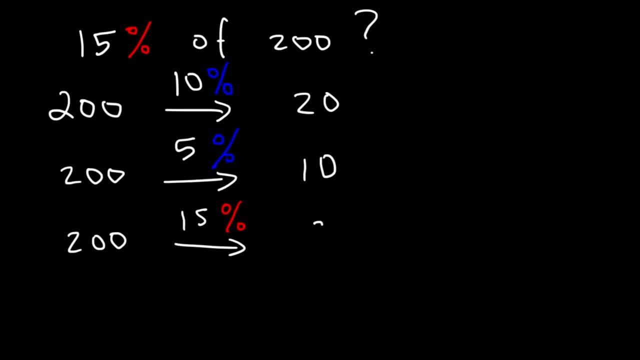 represent the value of 15% of 200, which is 30.. Now to confirm the answer using a calculator, here's what you need to do: Take 200 and multiply it by 15% as a decimal. To convert a percentage into a decimal, simply divide by 100. 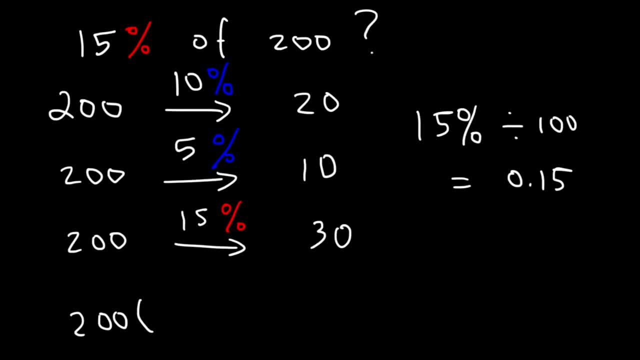 15 divided by 100 is 0.15.. You can also move the decimal point two units to the left. So those are two ways that you can use to convert a percentage into a decimal. Now let's multiply 200 by 0.15.. If you have a calculator, go ahead and 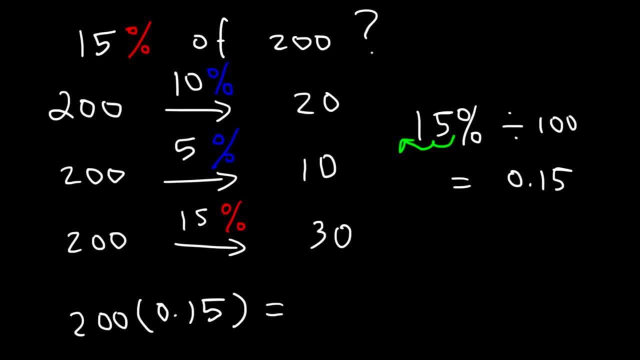 type this in, So 200 times 0.15 is indeed 350.. These are the two were data that can be used to match the data to a bin equal to 30. so now you know how to do percentages mentally, so let's go ahead. 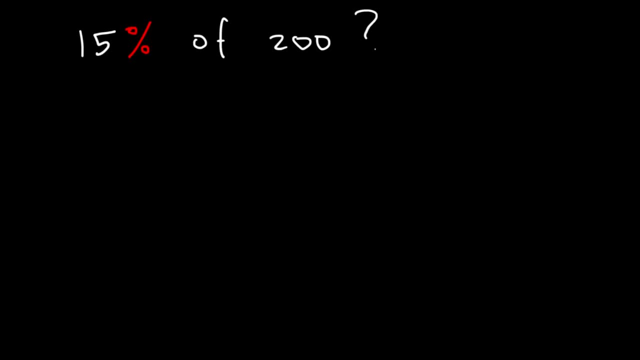 200?. How can we find the answer to this question mentally? Well, first ask yourself: what is 10% of 200?? To find 10% of a number, simply move the decimal one unit to the left. So 10% of 200 is 20.. Now, if 10% of 200 is 20,, what is 5% of 200?? 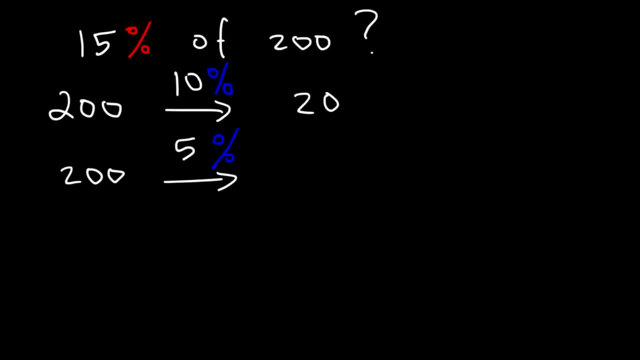 5% is half of 10%. So what is half of 20?? Half of 20 is 10.. So now, with this information, how can we find out the value of 15% of 200?? Well, since 10% plus 5% adds up to 15%, 20 plus 10 must. 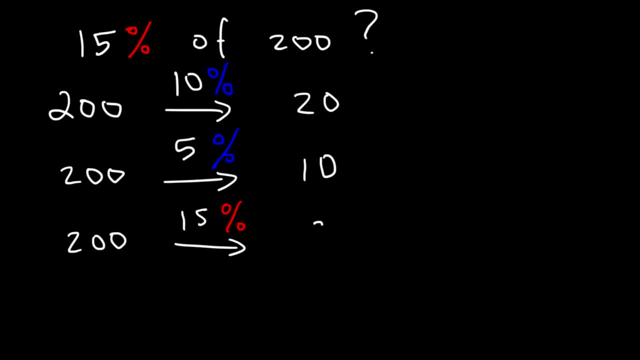 represent the value of 15% of 200, which is 30.. Now to confirm the answer using a calculator, here's what you need to do: Take 200 and multiply it by 15% as a decimal. To convert a percentage into a decimal, simply divide by 100. 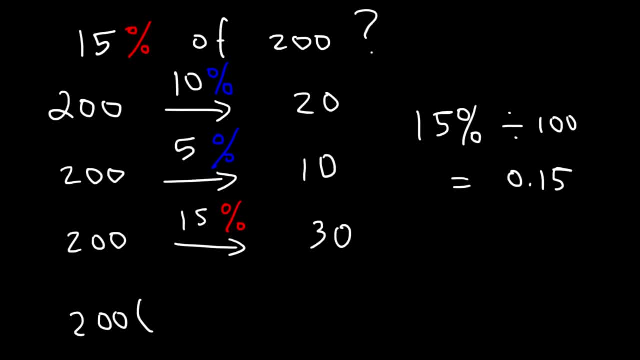 15 divided by 100 is 0.15.. You can also move the decimal point two units to the left. So those are two ways that you can use to convert a percentage into a decimal. Now let's multiply 200 by 0.15.. If you have a calculator, go ahead and type this in. So 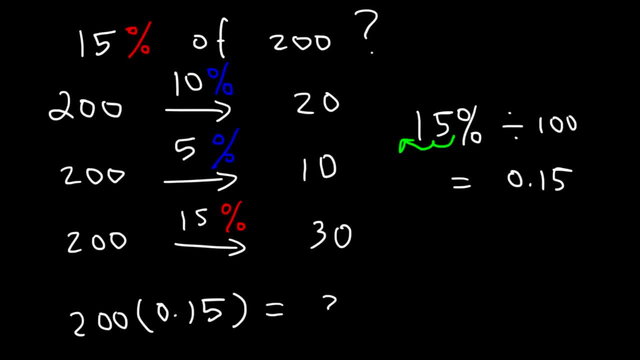 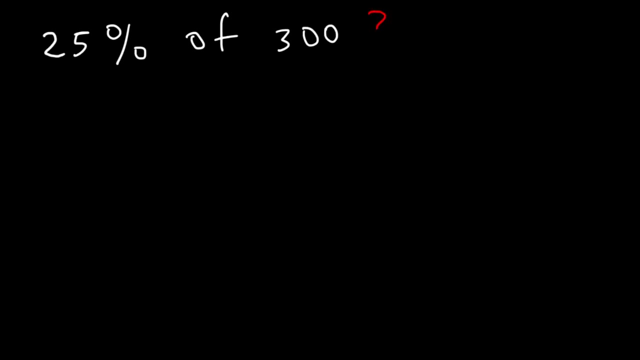 200 times 0.15 City & planned areas equal to 30. so now you know how to do percentages mentally, so let's go ahead and work on some more examples now. what is 25% of 300? go ahead and take a minute. 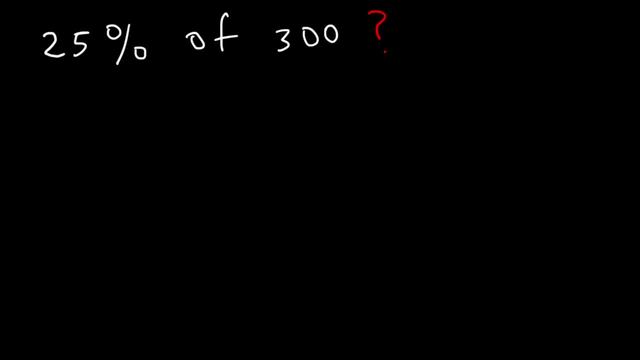 pause the video work on this example and then, once you have your answer, unpause it to see if you have the right answer. so let's start with 10% of 300. how much does that amount to? what is 10% of 300? 10% of 300 is simply 30. just move the. 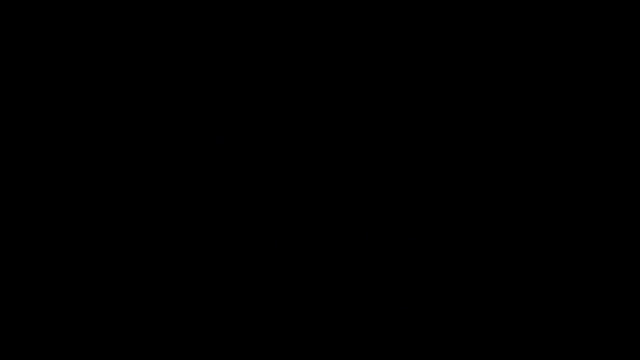 and work on some more examples. now, what is 25% of 300? go ahead and take a minute, pause the video, work on this example and then, once you have your answer, unpause it to see if you have the right answer. so let's start with 10% of 300. how much? 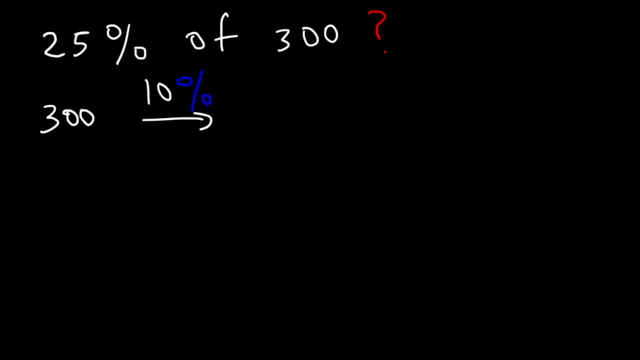 does that amount to what is 10% of 300? 10% of 300 is simply 30. just move the decimal one units left or take off a zero. so if that's 10%, how much is 20%? 20 percent is twice the value of 20%. 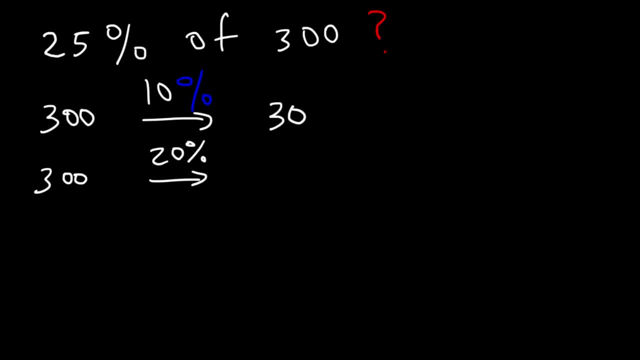 of 10%. so if we multiply 30 by 2, we're going to get 60. now to get to 25% we need to find the value of 5%. 5% is half of 10%, so half of 30 is 15. so now we 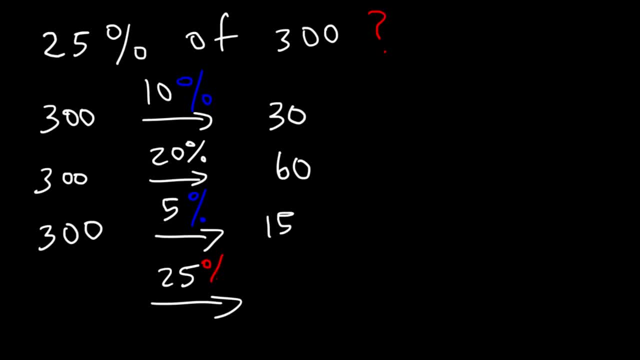 could find the value of 25%. 25 is the sum of 20 and 5, so therefore, to find the value of 25%, need to add 60 and 15. 60 plus 15 is 75. so now let's confirm this answer with the use of a calculator. let's multiply. 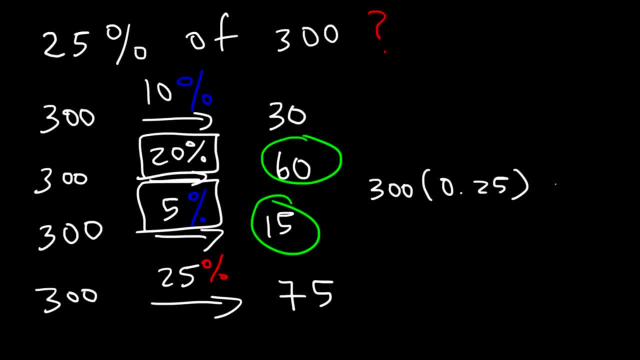 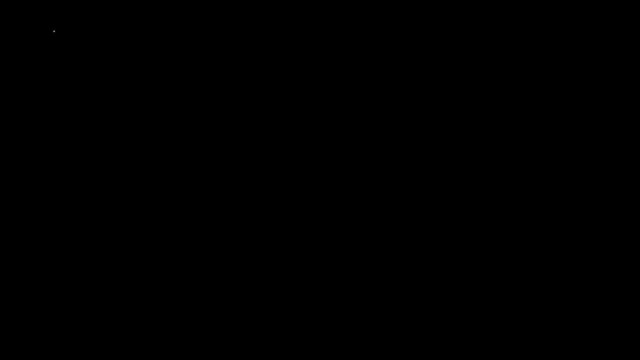 300 by 0.25, 25% as a decimal, and this will indeed give you 75. what is 40% of 500? go ahead and work on that question. so, as we've been doing before, let's start with 10%. so what is the value of 10% of 500? this is going to. 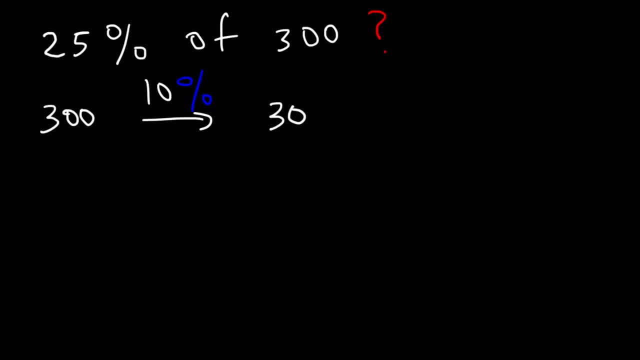 decimal, one units to the left or take off a zero. so if that's 10%, how much is 20%? 20% is twice the value of the answer. you have 10%. so if we multiply 30 by 2, we're going to get 60. now to get to 25%. 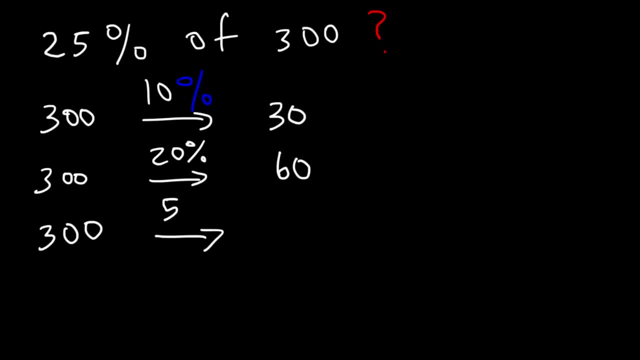 we need to find the value of 5%. 5% is half of 10%, so half of 30 is 15. so now we could find the value of 25%. 25 is the sum of 20 and five, so therefore, to find the value of 25%, we need to add 60 and 15, 60 plus. 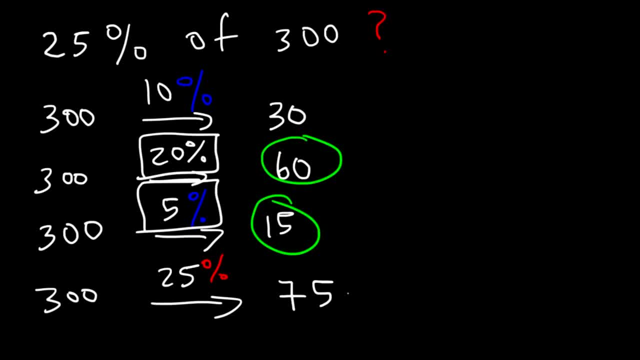 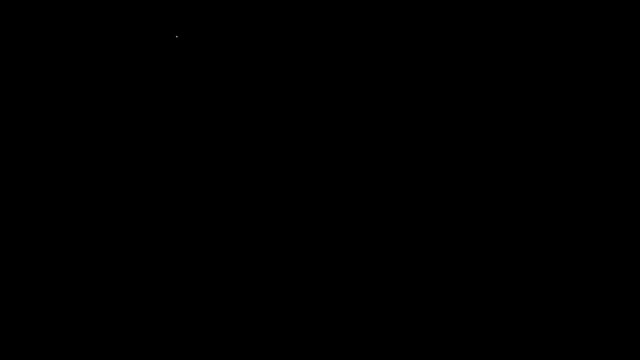 15 is 75. so now let's confirm this answer with the use of a calculator. let's multiply 300 by 0.25, 25% as a decimal, and this will indeed give you what is 40% of 500. go ahead and work on that question so, as we've been doing. 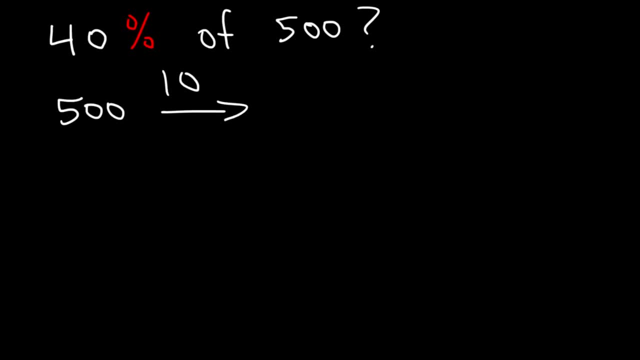 before. let's start with 10%. so what is the value of 10% of 500? this is going to be 50 if we drop off a 0, and now we could find 40%. 40% is simply 10% times. 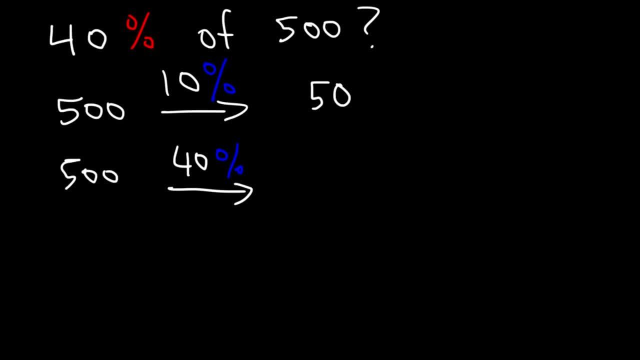 4. so if we multiply 50 by 4, what will that give us? so imagine if you have four $50 bills, you have basically 200. 4 times 0 is 0 and 4 times 5 is 20, so therefore 40% of 500 is 200. 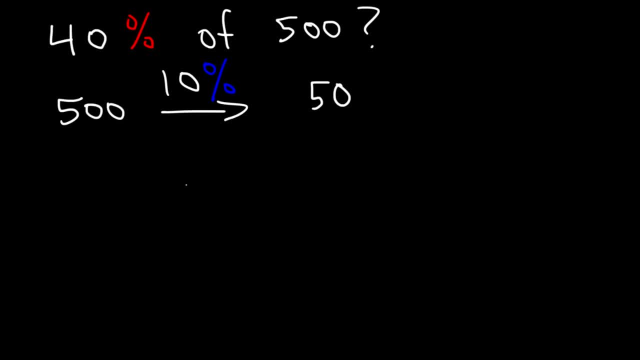 be 50 if we drop off a 0, and now we could find 40%. 40% is simply 10% times 4, so if we multiply 50 by 4, what will that give us? so imagine if you have four $50 bills. you have basically 200. 4 times 0 is 0 and 4 times 5 is 20, so therefore, 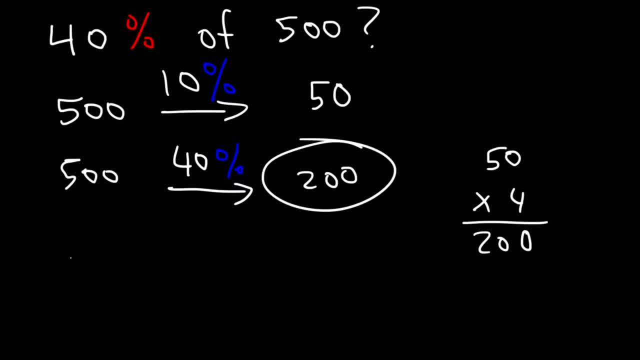 40% of 500 is 200, and if you multiply 500 by point 4, this will also give you 200 as well. now let's move on to our next example. what is 24% of 80? so let's make it a little bit more. 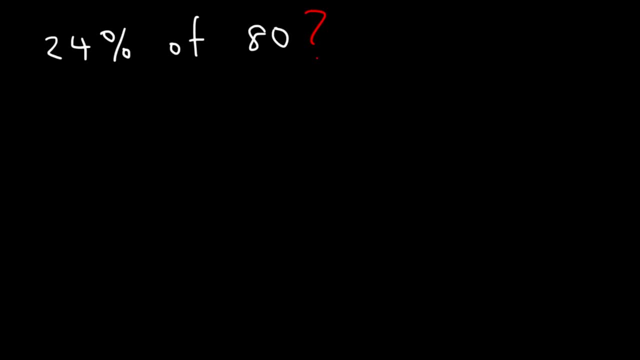 challenging. go ahead and try that. so first let's calculate 10% of 80. 10% of 80 is 8, and 20% of 80 is basically 8 times 2, that 16. now we need to get to 24%. so it's helpful if we find the value. 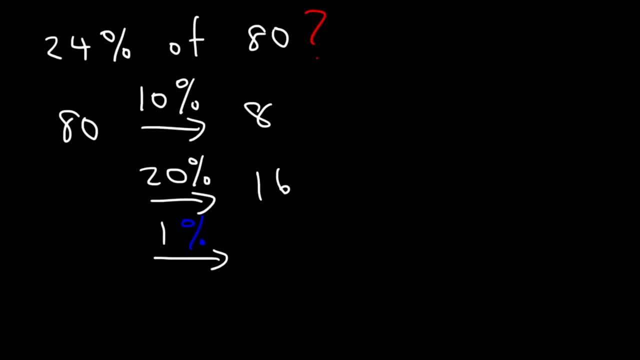 of 1%. if 10% is 8, then 1% is .8. basically move the decimal one unit to left, or divided by 10. so if 1% is .8, what is the value of 4%? well, if 8 times 4 is 32. 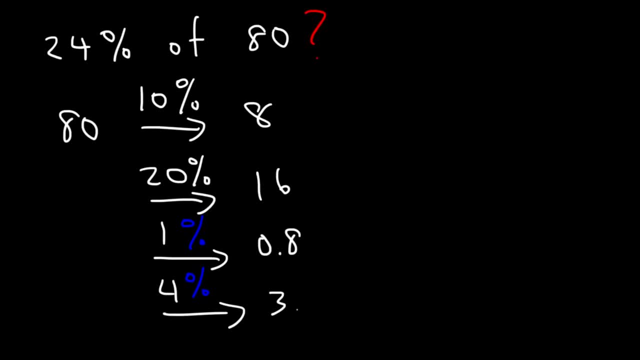 and then .8 times 4 must be 3.2. now to get to 24% we need to add 20% and 4%. so basically we need to add 16 and 3.2. so 16.0 and 3.2, 2 and 0 is 2, 3 and 6 is 7. 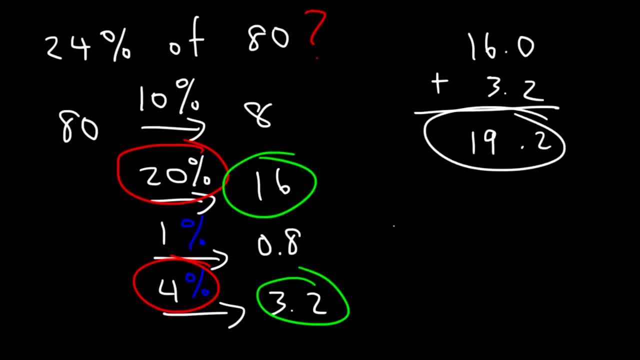 and 6 is 9, so it's 19.2. so if we multiply 80 by .24, this will give us 19.2. so you can always check your answer with the use of a calculator to make sure you're doing it right. 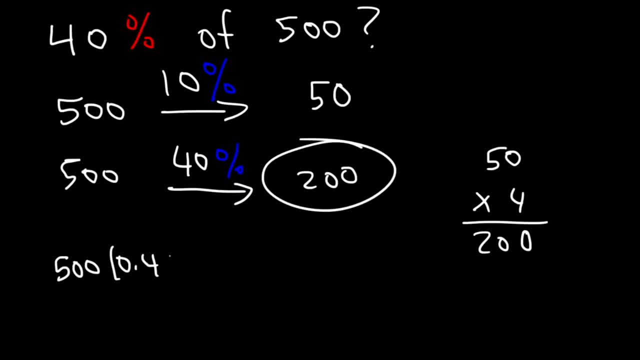 and if you multiply 500 by point 4, this will also give you 200 as well. now let's move on to our next example. what is 24% of 80? so let's make it a little bit more challenging. go ahead and try that. 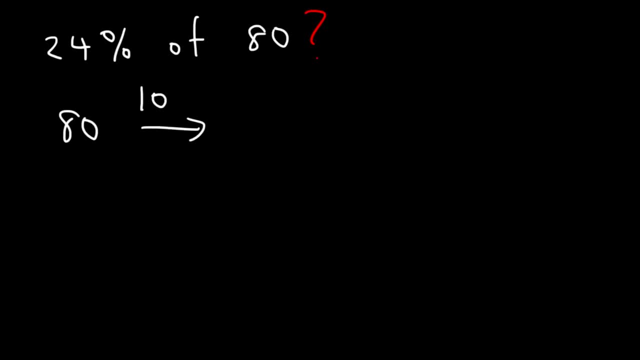 so first let's calculate 10% of 80. 10% of 80 is 80, and 20% of 80 is basically eight times two, that's 16. now we need to get to 24%. so it's helpful if we find. 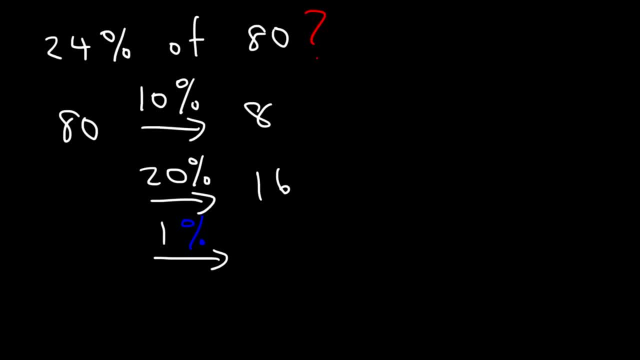 the value of one percent. if 10% is a, then one percent is 0.8. basically move the decimal one unit to left or divided by 10.. So if 1% is 0.8, what is the value of 4%? 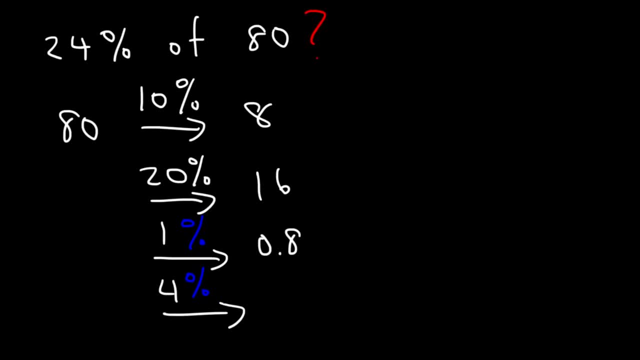 Well, if 8 times 4 is 32, then 0.8 times 4 must be 3.2.. Now to get to 24%, we need to add 20% and 4%. So basically we need to add 16 and 3.2.. 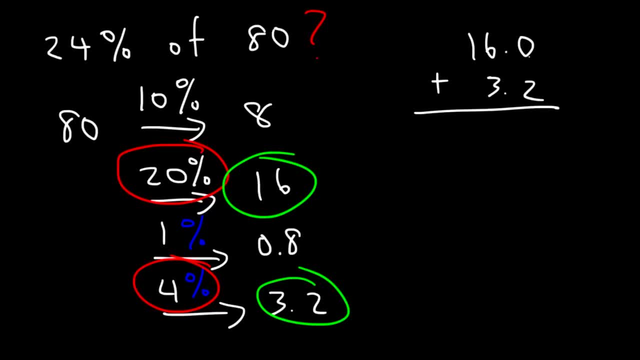 So 16.0 and 3.2,, 2 and 0 is 2,, 3 and 6 is 9, so it's 19.2.. So if we multiply 80 by 0.24,, this will give us 19.2.. 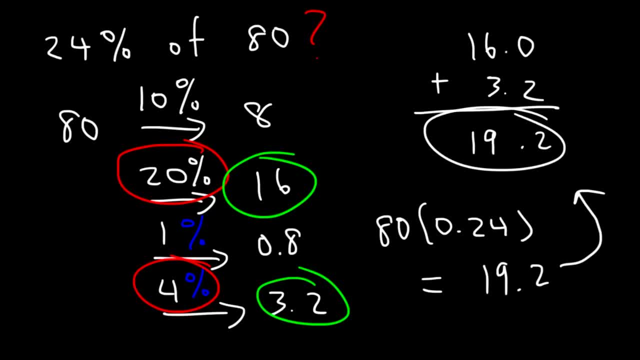 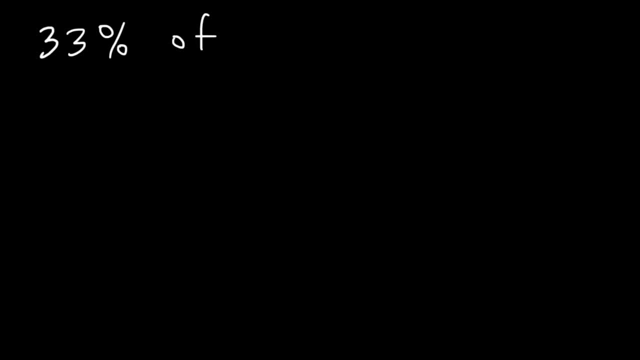 So you can always check your answer with the use of a calculator to make sure you're doing it right. What is the value of 32?? It's 33% of 120.. So now that you know how to do the last example, you can do this one. 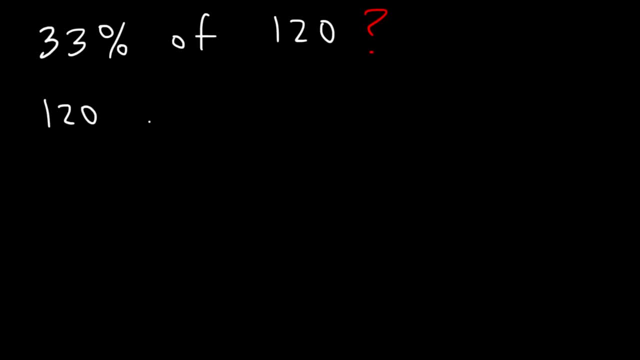 So go ahead and try it. So, as always, I'm going to start with 10%, since that's a nice number to deal with. So what is 10% of 120?? Well, if we drop off the 0,, 10% is going to be 12.. 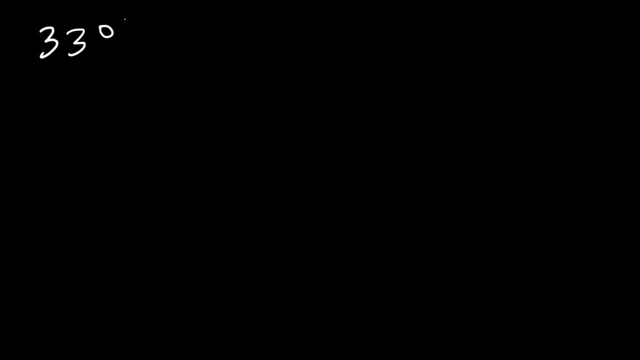 what is the value of 33%, of 120? so now that you know how to do the last example, you can do this one, so go ahead and try. so, as always, I'm going to start with 10%, since that's a nice number to. 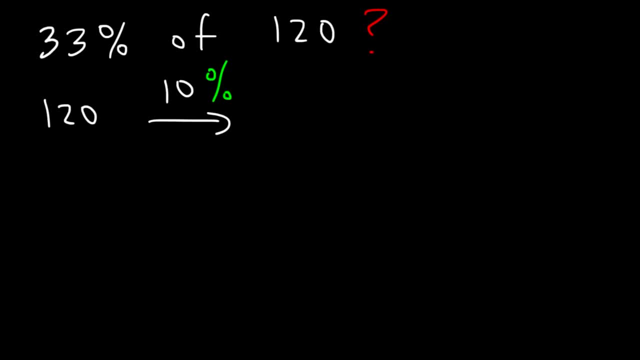 deal with. so what is 10% of 120? well, if we drop off the 0, 10% is going to be 12. now we need to find 30%. our goal is to get up to 33%. 30% is 3 times the value of 10%. 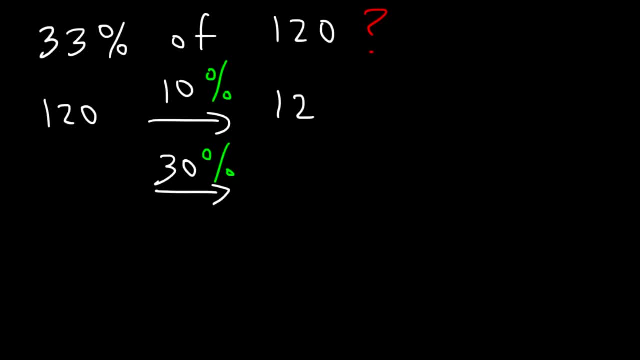 10 times 3 is 30. so if 10% is 12, then 30% must be 12 times 3, which is 36. now our next thing that we need to find is 1%. if we could find the value of 1%, we 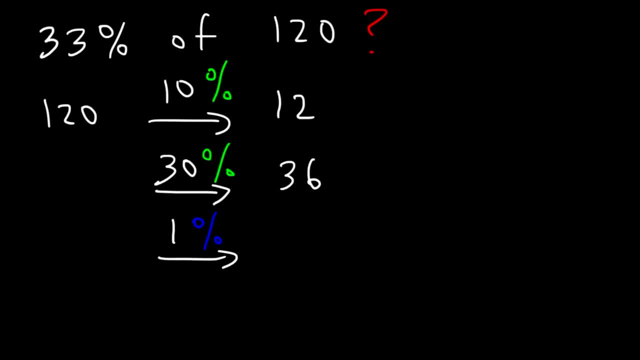 could find the value of 3%. now if 10% is 12, 1% is basically 12 divided by 10 or 1.2. just move the decimal one unit to the left. so 3% is going to be 3 times 1.2, because 3% is 3 times 1%. now if 12 times, 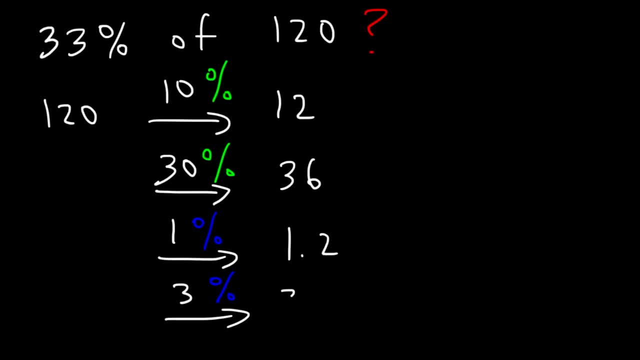 3 is 36, then 1.2 times 3 must be 3.6. since we're looking for 33%, we need to add 30% plus 3%, so we need to add 36.0 plus 3.6. 6 plus 0, 6, 3 plus 6 is 9, so it's. 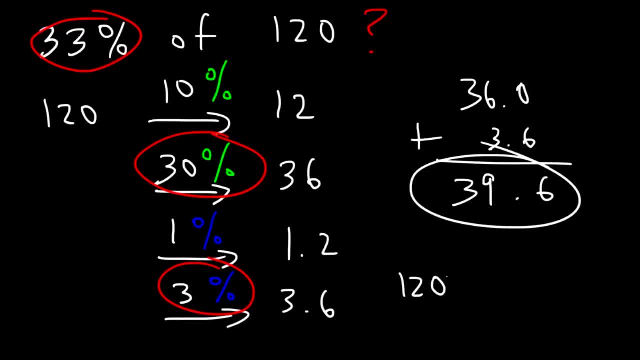 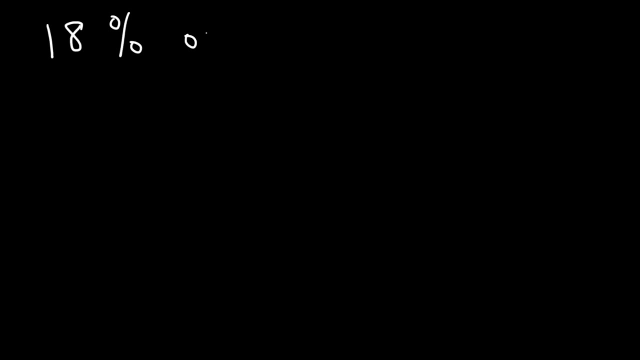 39.6. and now let's confirm it. let's multiply 120 by 0.33, this is equal to 39.6. so that's the same answer as what we have here. now, what is 18% of 39 so 39.6? so let's say 18% of 39 is equal to 39.6. so let's say 18% of 39 is equal to. 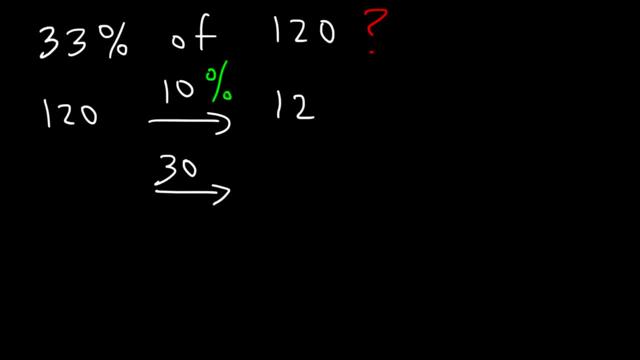 Now we need to find 30%. Our goal is to get up to 33%, So we're going to do that. 30% is 3 times the value of 10%. 10 times 3 is 30. So if 10% is 12, then 30% must be 12 times 3,, which is 36.. 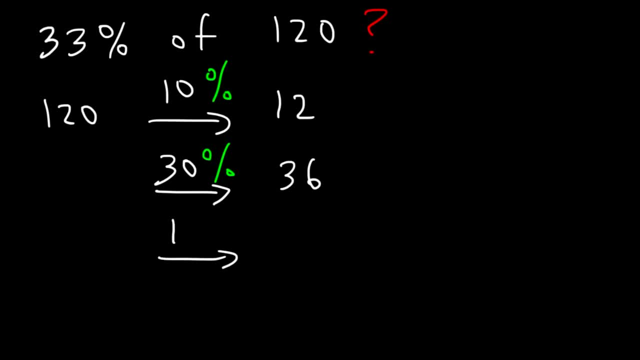 Now our next thing that we need to find is 1%. If we could find a value of 1%, we could find a value of 3%. Now, if 10% is 12,, 1% is basically 12 divided by 3.. 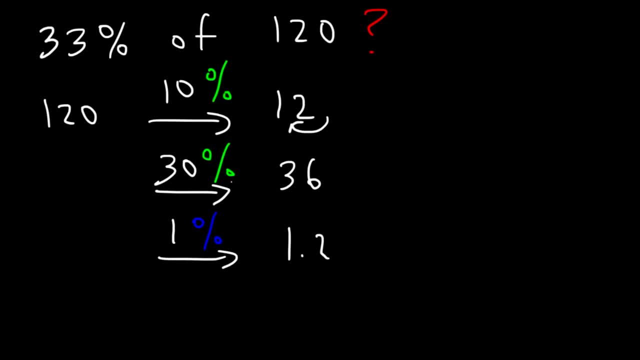 So we can just move the decimal one unit to the left. So 3% is going to be 3 times 1.2, because 3% is 3 times 1%. Now if 12 times 3 is 36, then 1.2 times 3 must be 3.6.. 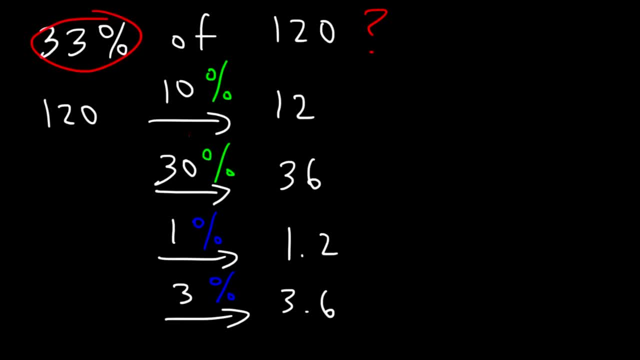 Since we're looking for 33%, we need to add 30% plus 3%. So we need to add 36.0 plus 3.6.. 6 plus 0 is 6.. 3 plus 6 is 9.. 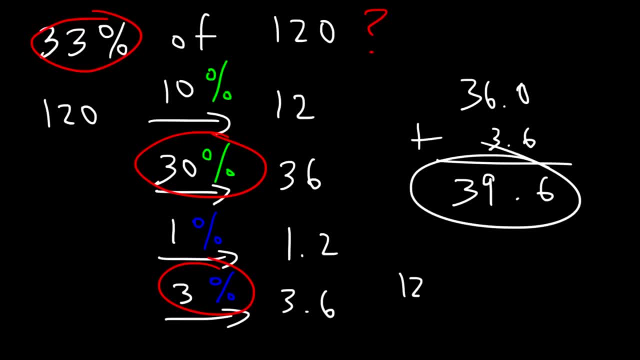 So it's 39.6.. And now let's confirm it. Let's multiply 120 by 0.33.. This is equal to 39.6.. So that's the same answer as what we have here. Now, what is 18%? 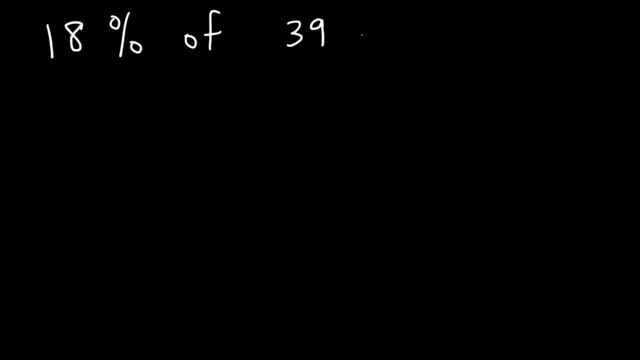 Of 39. So let's say, if your restaurant bill comes to $39 and you want to make an 18% tip, What is the value of the tip? How much should you pay in tips? So first let's find the value of 10%. 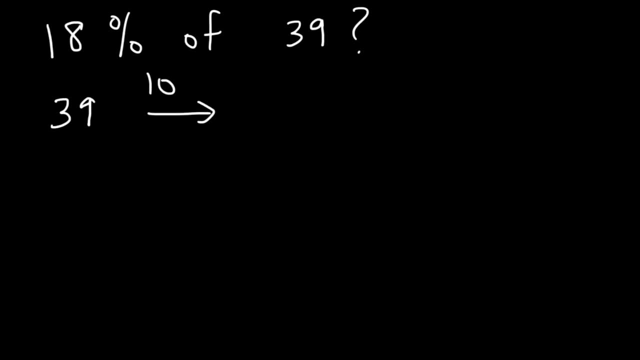 Our goal is to get a total of 18%. 10% of 39 is 3.9.. Now let's find the value of 5%. 5% is half of 10%, So what is half of 3.9?? 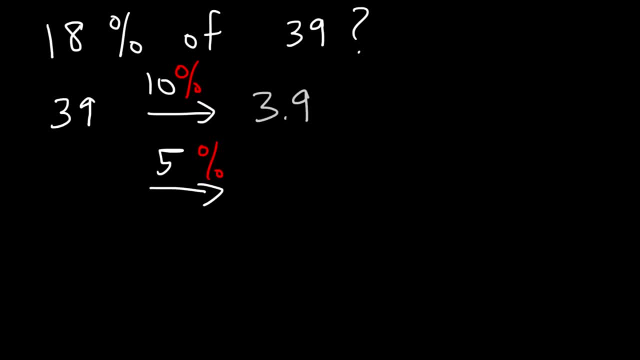 Well, let's say, if you have $3.90, you want to split it two ways: To split $3.00 evenly, it's basically $1.50. And to split 90 cents evenly, it's 45 cents. 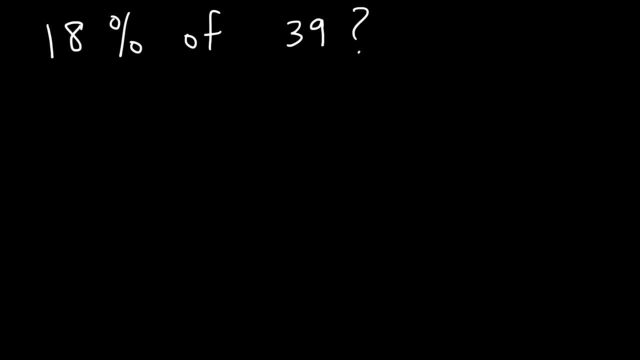 gorillas. ok, let's say 18.3早が, all right, all right. let's first look at entry about what's the value. of our focus is the cost of editing so we can see if your restaurant bill comes to $39 and you want to make an 18% tip, what is the 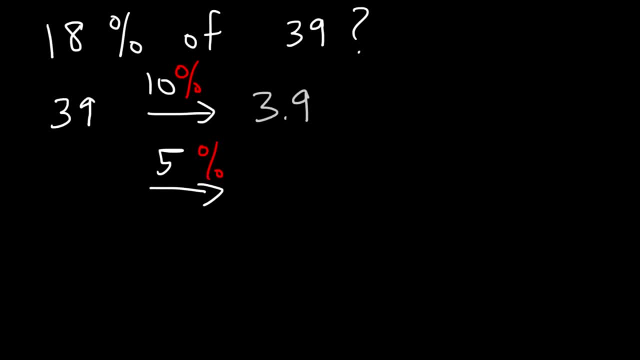 value of the tip. how much should you pay in tips? so first let's find a value of half of 3.9. well, let's say, if you have three dollars and ninety cents, you want to split it two ways. to split three dollars evenly, it's basically a buck. 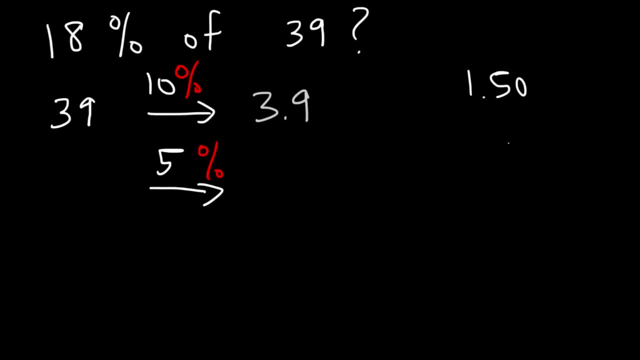 fifty and to split in ninety cents evenly, it's 45 cents. so if you add these two, it's a dollar ninety-five. so half of 3.9 is 1.95. now what about 1%? if 10% is 3.9, 1% is 0.39. now we need 3%, because 15 plus 3 adds up to 18. so let's. 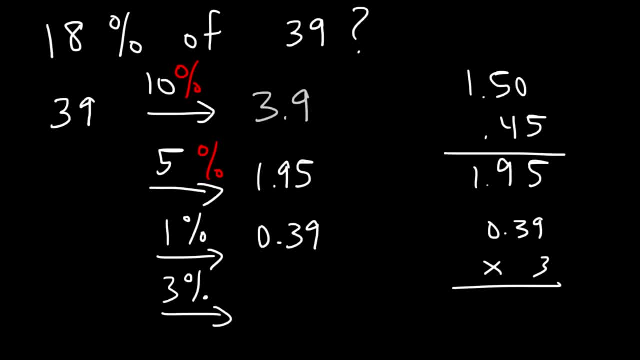 multiply 0.39 by 3, so 3 times 9 is 27 and 3 times 3 is 9 plus 2, that's 11. so this is what we have now. where should we put the decimal point? we only have two. 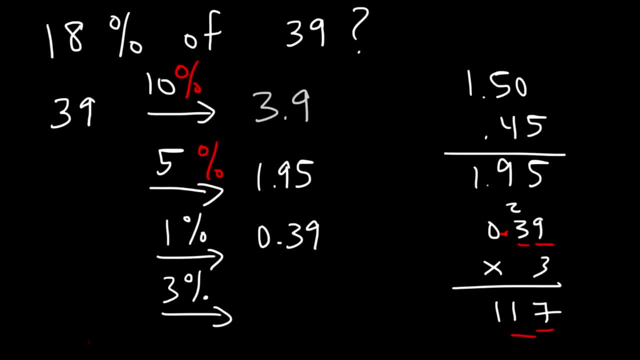 digits to the right of a decimal point, so that has to be the same. therefore, the decimal point is going to come after the first one. so 39 cents times 3 is basically a dollar 17. so now what we need to do is we need to add 10% plus 5% plus 3%, because that's 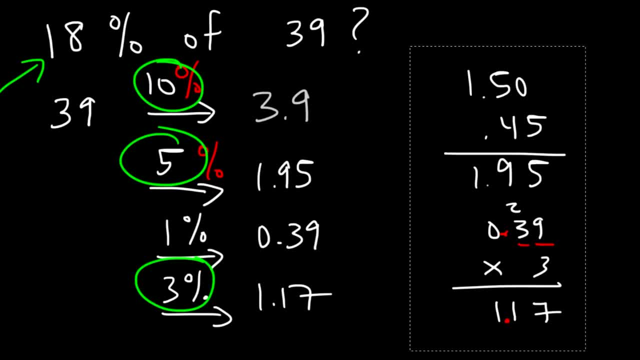 going to add up to 18%. so let's add 3.9, 1.95 and 1.17, so 5 plus 7 is 12. 1 and 9 is 10. 9 and 1 is 10, so that's 20. we're. 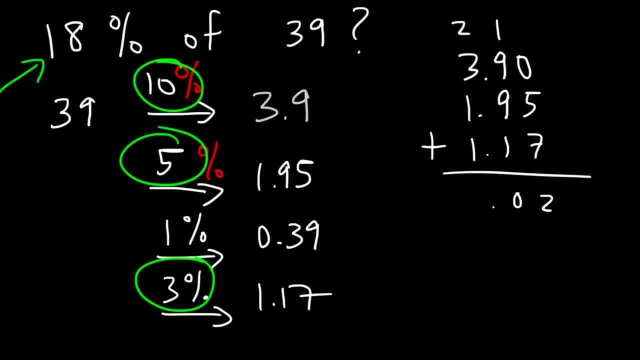 going to write a 0 and then put a 2 here. 2 plus 3 is 5 plus 1 is 6, plus 1 is 7. so it's seven dollars and two cents. now let's confirm the answer with the calculator: 39 times 0.18.